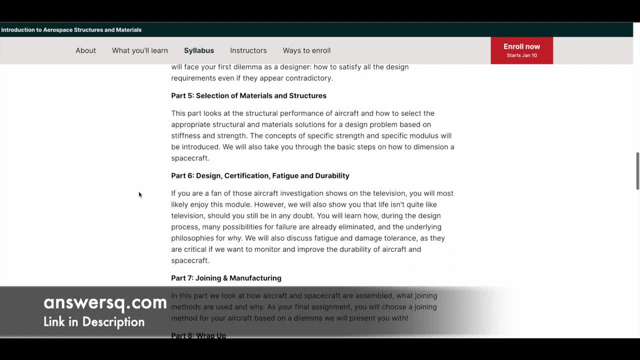 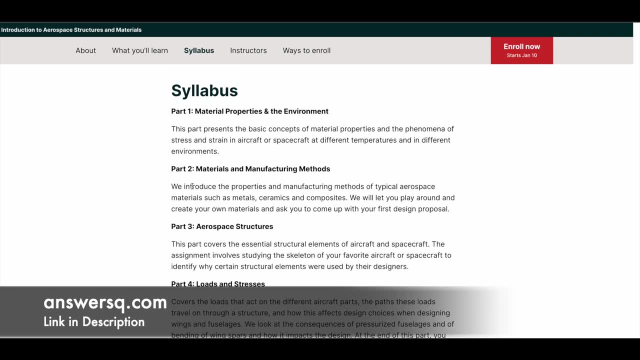 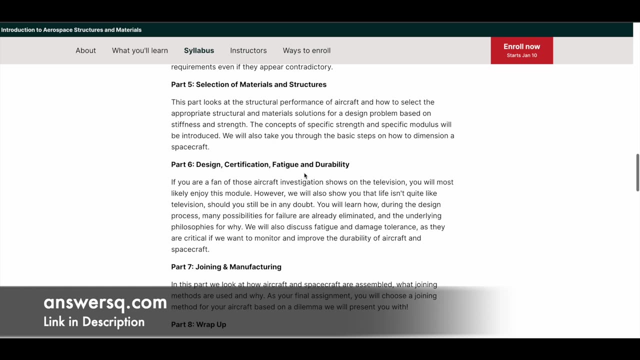 you are going to learn. So they have divided this course into eight parts, starting with material properties and the environment, And the second part is materials and manufacturing methods, aerospace structures, loads and stresses, selection of materials and structures, design, certification, fatigue and durability. And you can see you have two more lessons. 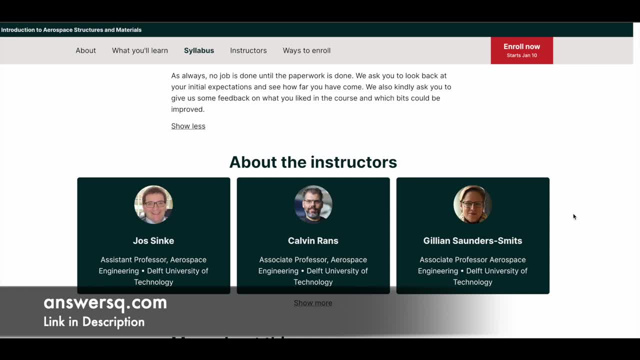 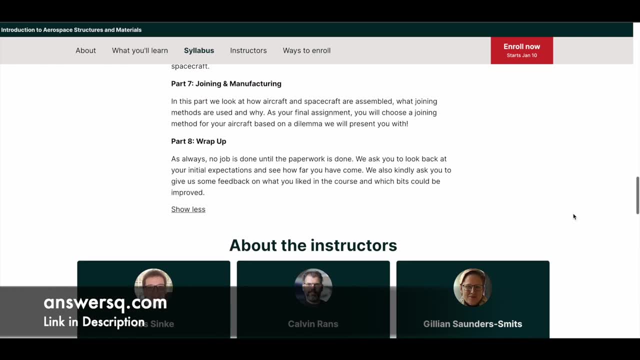 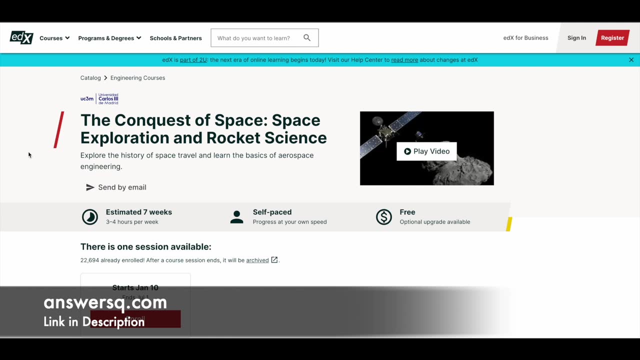 And these people are going to teach you about aerospace engineering And these are the people who are teaching and delft university of technology. So you are going to learn from people have very good experience in this field. So this is the first one. make use of it. next one is the conquest of space. 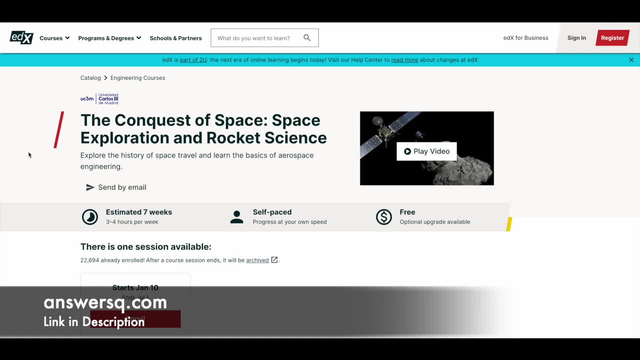 Space exploration and rocket science. So in this program You will get to learn about the history of space travel and you learn more basics of aerospace engineering. Next one is also offered by TU delft, which is introduction to aeronautical engineering In the. in this program you will learn about the science behind flying. 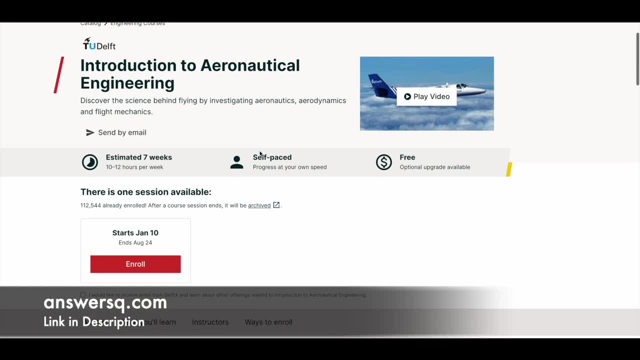 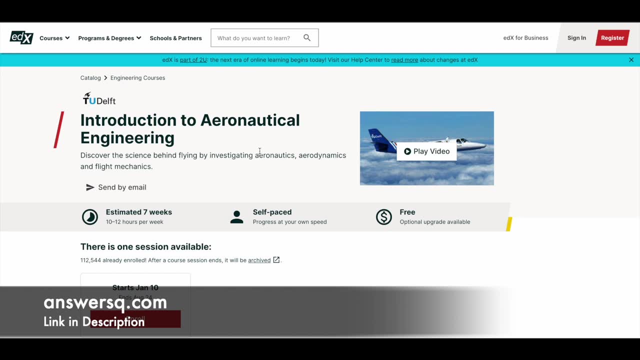 By investigating about aeronautics, aerodynamics and flight mechanics, and more things will be covered. So this is a bit of long course. It takes approximately seven weeks to complete this course, Even if you spend 10 to 12 hours per week and you can just scroll down and see what. 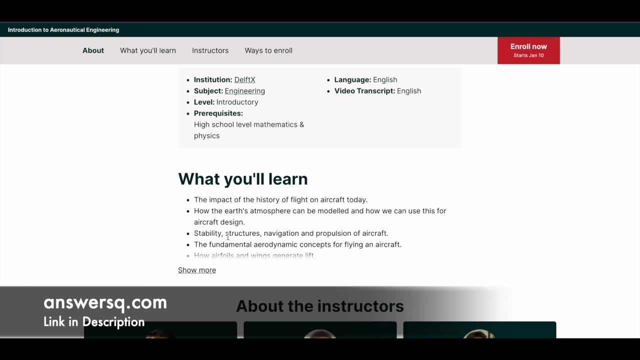 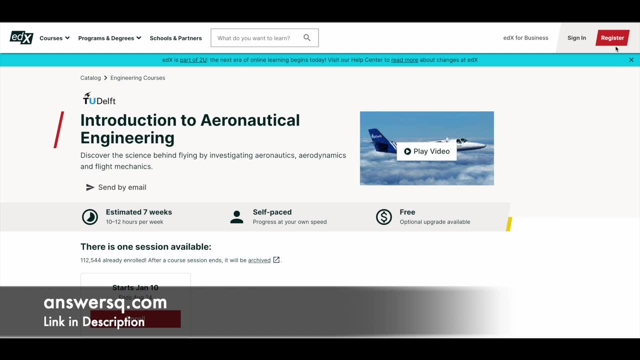 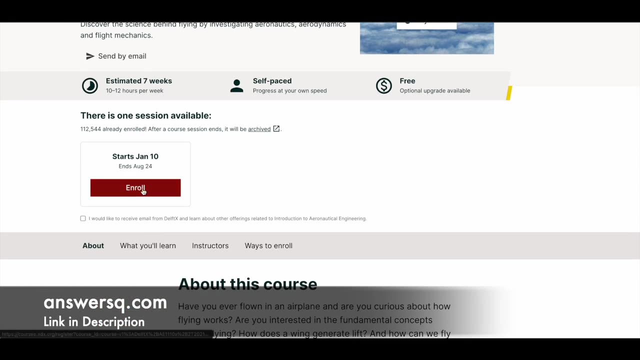 Exactly will be covered in this course, Here, and what you learn, and instructors. everything will be given in the course page. just go through it. So now to enroll in these courses, You can simply click on register and log into your edX account And then, once you are logged into your account, just click on this enroll button that you see here. 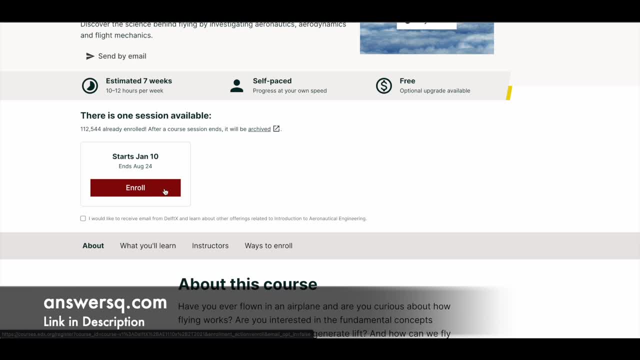 And then you will see two options. one is to take the course for free and the other one is a Verified track in which you have to pay and enroll the enroll in the course. So if you go for the paid track, you can get the certificate. if you go for the free track, 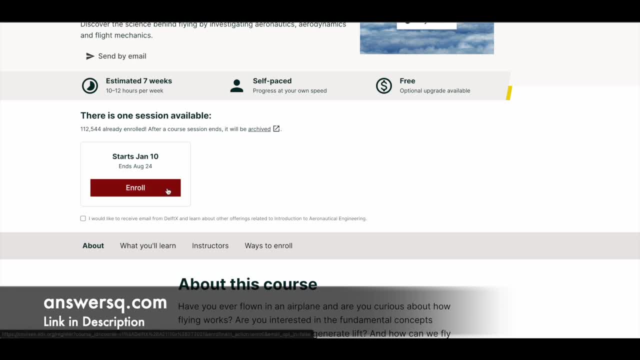 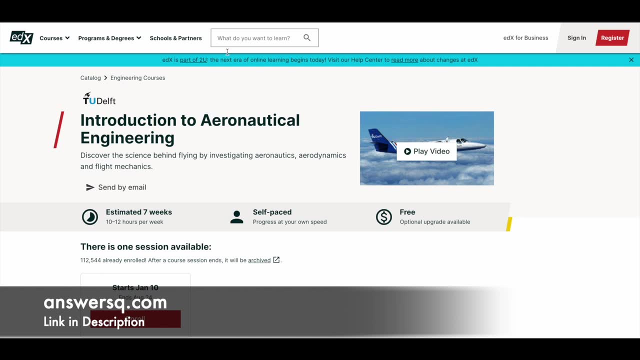 You can learn, But you will not get the certificate. so it's up to you. You can choose whichever track you want, but you can learn for free. that is option. So these are the three courses that are available in edX. Next one is rocket science- physics. first principles from SpaceX. 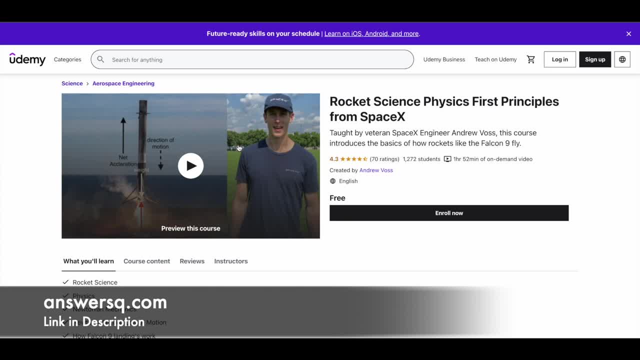 So this program is taught by Andrew was, who has worked in SpaceX as an engineer, So it's a short course. It's a two-hour course in which you will get to learn about rocket science and the physics behind it, and You will get to learn more about these things in this course, which is offered by one of the X SpaceX engineer. 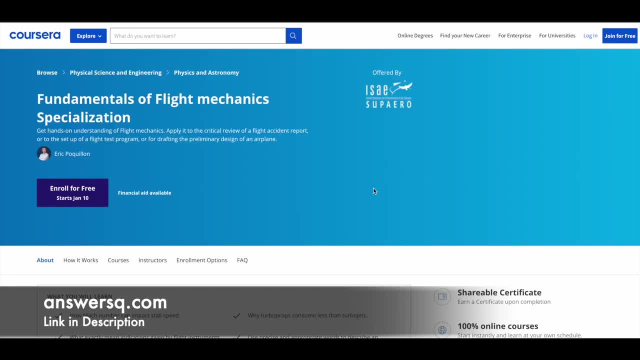 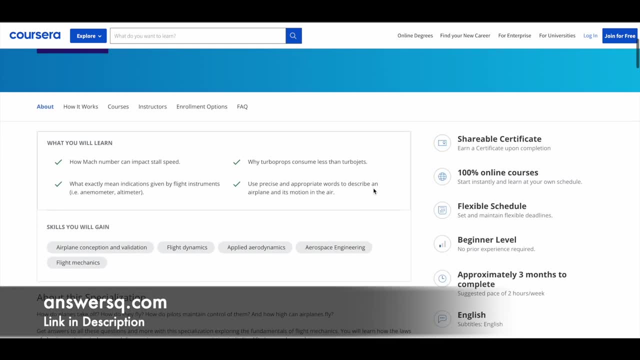 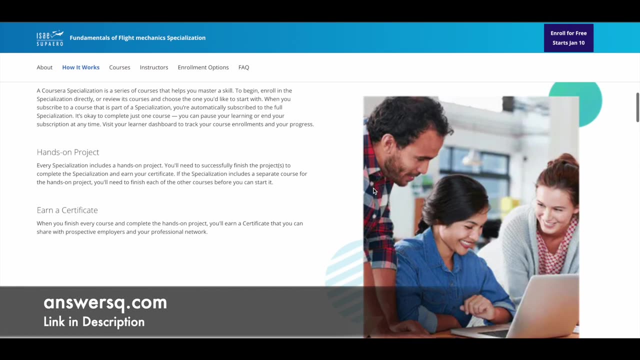 Next one is fundamentals of flight mechanics specialization, which is available in Coursera. So in this program you will get to learn about airplane conception and validation, flight dynamics, applied aerodynamics, aerospace engineering, flight mechanics and lot more, and You have four courses in this specialization. 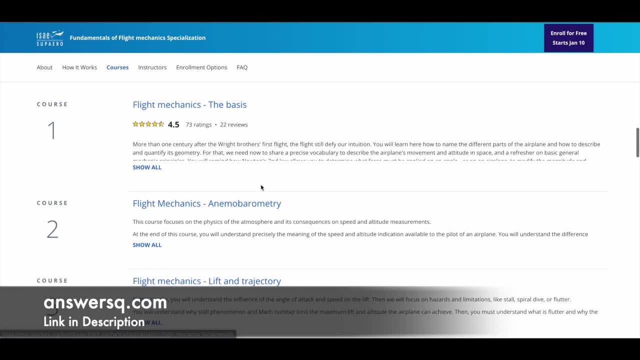 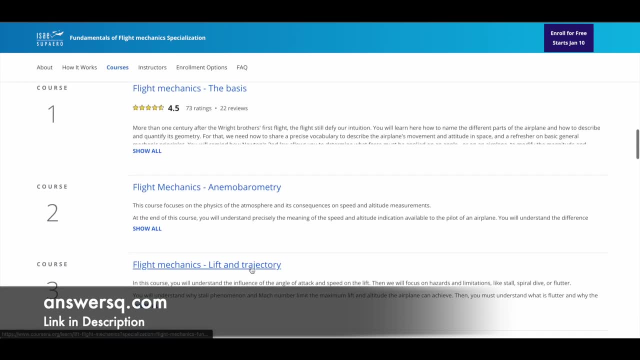 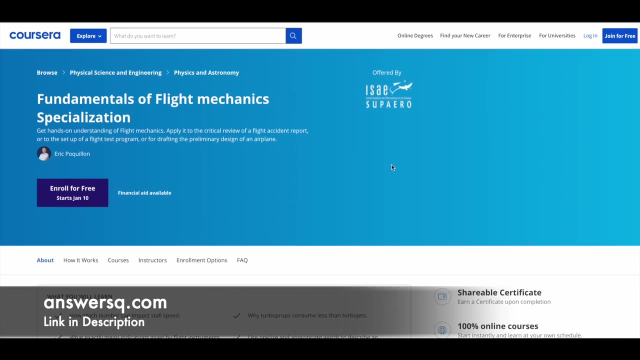 so of course now One is flight mechanics, the basis, and you can see here There are a few more courses. totally We have four courses, as as it is mentioned here. So now let me tell you how to get the courses for free in Coursera. So this is a specialization page, or you will probably land on this page after you click on the link. 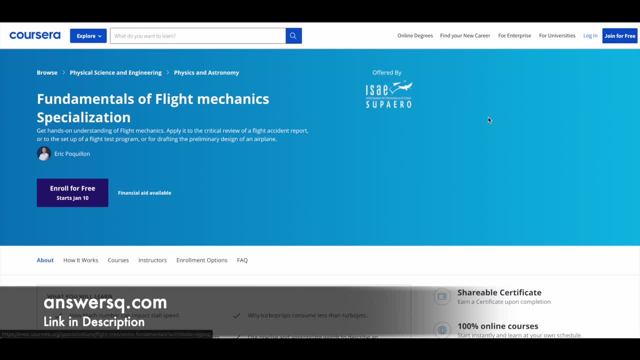 Which I'll be giving you. so what you have to do is just click on join for free and and log into your Coursera account And once you are logged in, if you just click on this enroll for free from the specialization page, You will not see any. 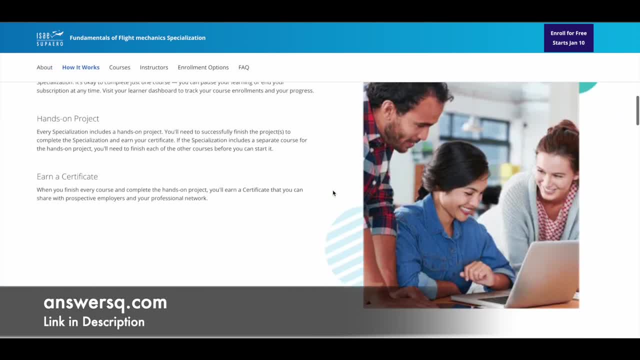 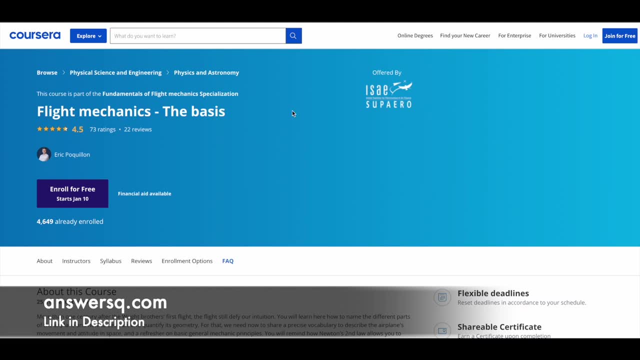 Option to enroll in the course for free. So what you have to do is you have to open the individual courses. Just click on the course title here and you will be directed to the course page and from here, If you just click on enroll for free, a pop-up will appear and then you will see at the bottom, audit the course. 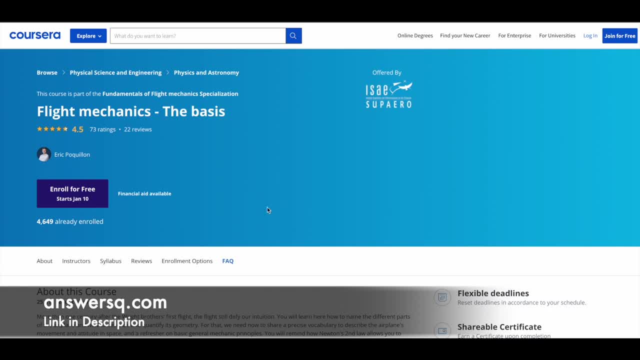 If you just click on audit, you will be automatically enrolled in the course and you can start learning for free. So the important thing to note here is you can learn for free. All these courses have an option through which you can enroll in the program for free and learn for free. 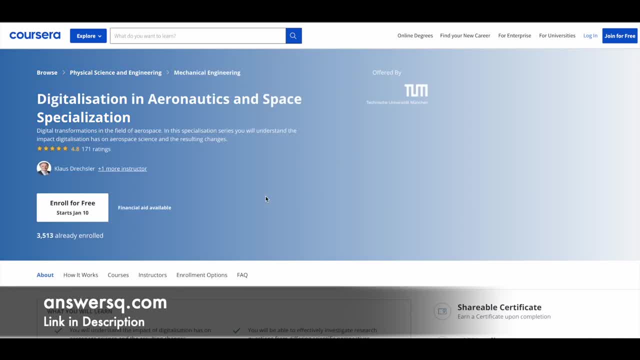 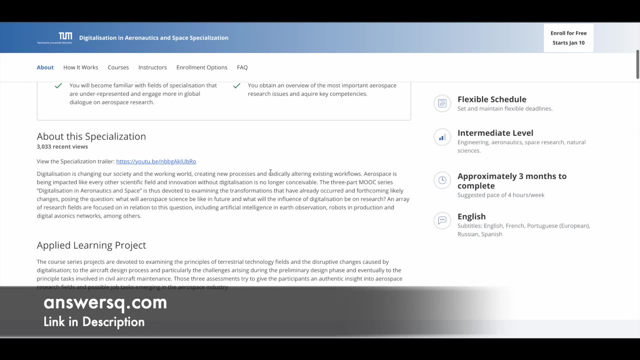 So next one in the list is digitalization and aeronautics and space Specialization, and this is taken by one of the most popular universities in Germany, So the content will be very good again in these programs. make use of it. All these programs are given by top instructors and top universities around the world.